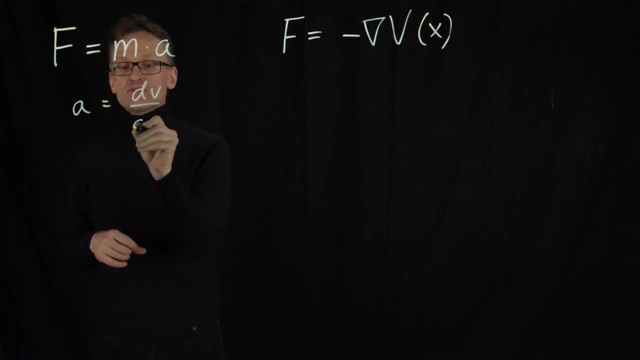 Acceleration. in turn, that was the derivative of the velocity with respect to time And that means that if I knew the previous velocity, I can calculate how the velocity is changing. And if I know that velocity, I know that velocity is the derivative of position as a. 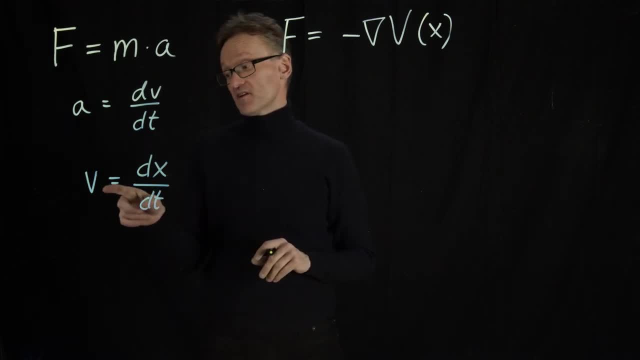 function of time. So if I knew some starting positions here and I know the velocities, I can calculate the new positions. And if I now have new positions then I just go back here, plug those new positions in my potential and force and then I keep repeating this for many time. steps. 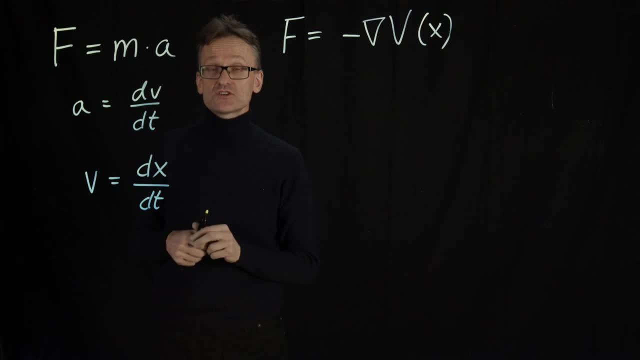 And if I do this and if I have accurate starting positions, I need to know the starting velocities too. I can just predict the exact motions, paths, trajectories individual atoms will take. There are a couple of problems with that, though. First, 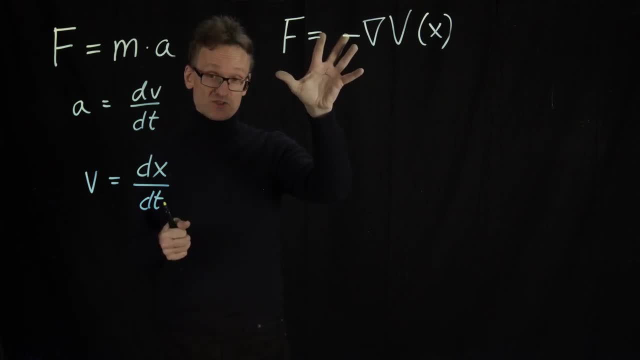 this is going to involve some of the simplified potentials we used we defined in Lecture 1.. They're not perfect. Second, we do not know the starting positions exactly, Starting velocities. there is certainly no database where you can get that, So you're going to need to assign velocities. 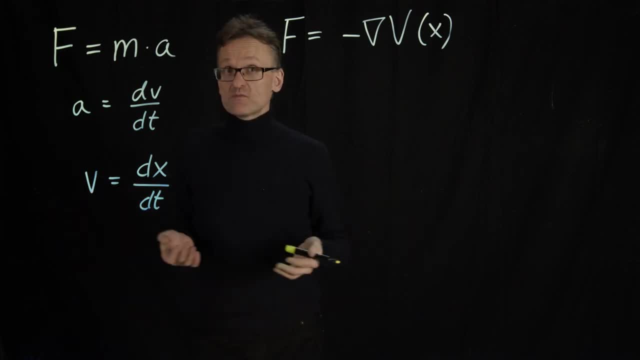 maybe from the Maxwell-Boltzmann distribution. That's what I would normally do, But they're going to be random And depending on the velocities you pick, you will have different paths here. That's going to start to sound a bit strange. The other problem is that, even if 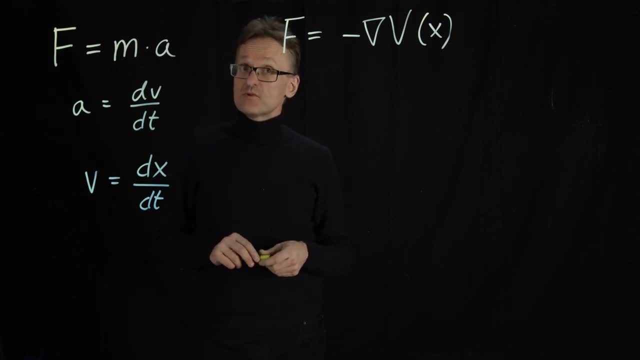 you knew all these things perfectly when you start. the problem is that a computer not perfect the computer. actually we're using floating point numbers, 32 bits, 64 sometimes, to treat this and that means that there is a finite resolution to the calculation done by the computer. 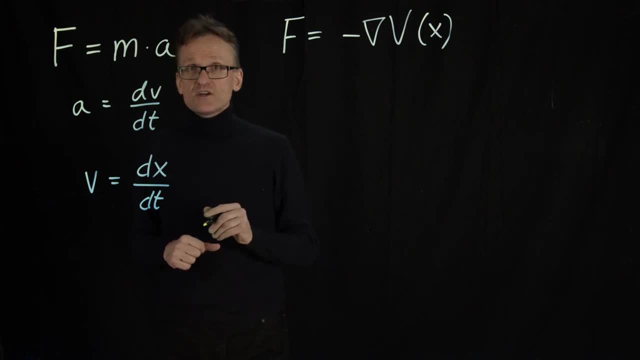 these systems are differential equations with many, many, many degrees of freedoms, and you can even show that they have so-called positive Lyapunov exponents. they are chaotic. what that means? that if I start with the system, if I start with the, say exactly the same starting condition. 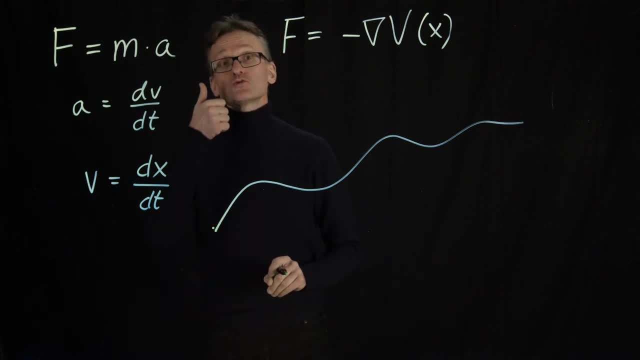 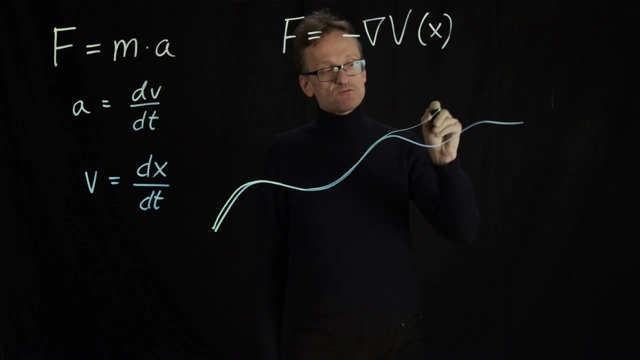 and then I introduce an exceptionally small error. I'm taking just one bit in the computer. initially these trajectories are going to follow each other very closely, but eventually those differences will grow and at some point I'm going to take a completely different path. so based on that, we